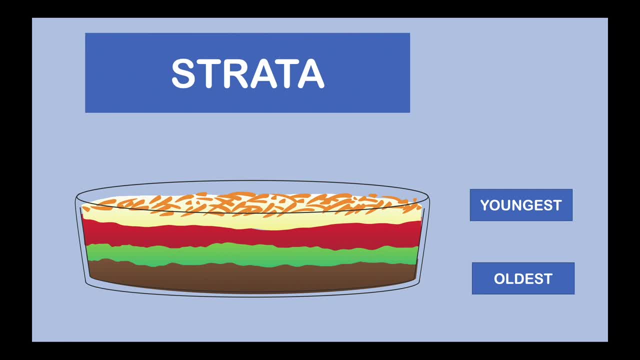 Cheese is your youngest layer. Scientists call each one of these layers in rocks strata, So let's call them strata in our bean dip too, Why not? It's a party for scientists. Stratigraphy is the scientific study of layers, and that's usually something that we study in rocks. And if you want, 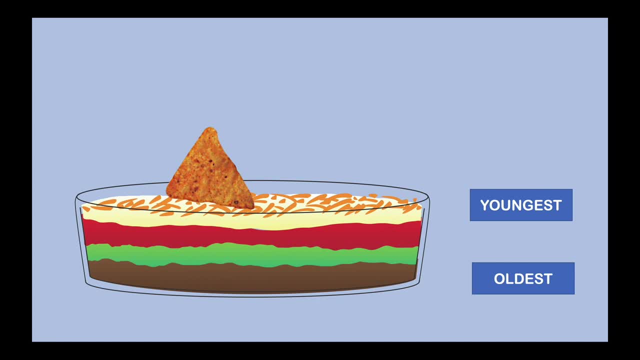 to really impress people at your party. while you're eating your tasty five-layer bean dip, you can tell them that this bean dip preserves the law of superposition. That means that the newer layers form on top of previous layers. Either way, let's eat. If you go someplace like the Grand Canyon where there are a lot of layers, 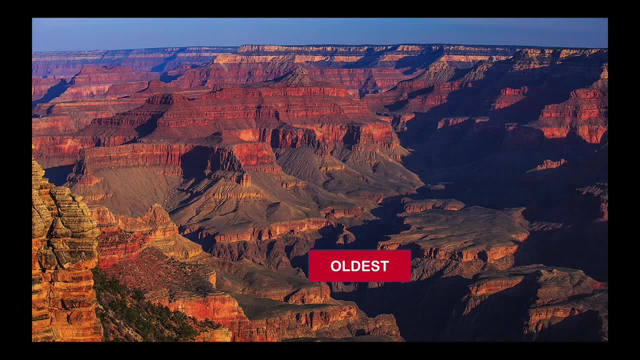 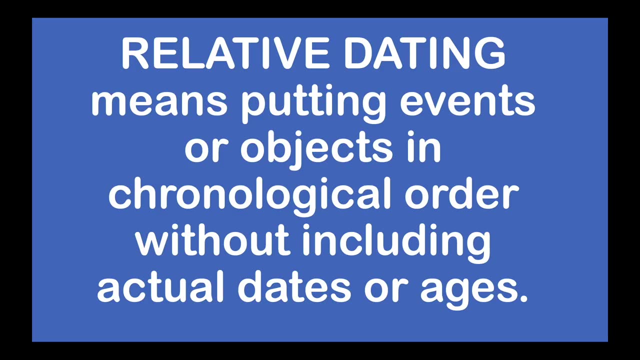 in our earth that are exposed, you'll see that the oldest layers are found at the bottom and the youngest layers are found at the top. So relative dating means putting events or objects in chronological order without including events or objects in chronological order, without including events or objects in chronological order without including 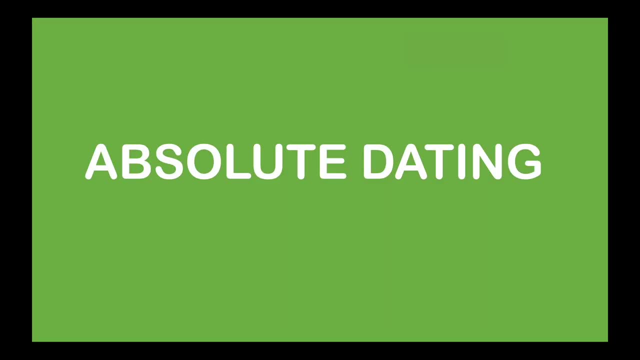 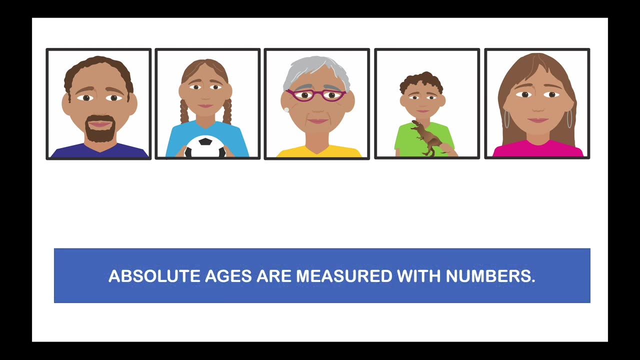 actual dates or ages, But absolute dating is a little different. Let's go back to our family again. Absolute ages are measured with numbers. So if we want to measure the absolute age of each one of these family members, we could look at their birth certificates and we'd find that mom 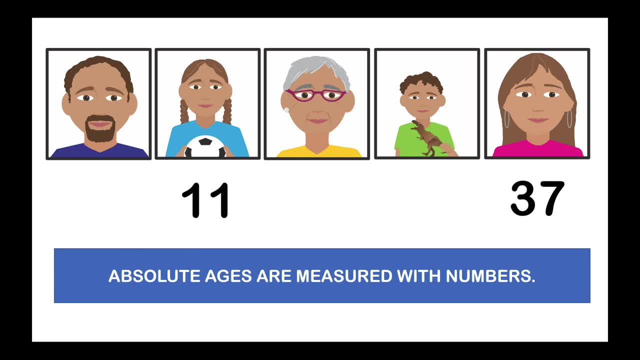 is 37, and the daughter is 11,, the little boy is 7,, dad's 39, and grandma? well, she's not going to tell you how old she actually is. She prefers relative dating because, like a lot of grandmas, she doesn't really want to say her age in numbers. 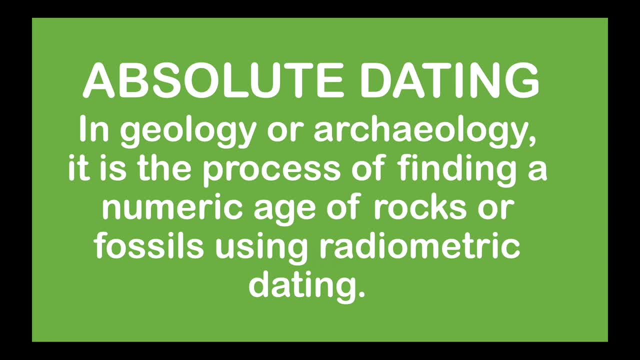 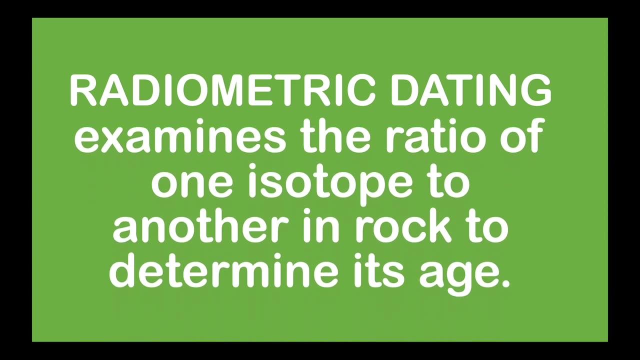 Absolute dating in geology or archaeology is the process of finding a numeric age of rocks or fossils using radiometric dating. So what is radiometric dating? Radiometric dating examines the ratio of one isotope to another. Radiometric dating examines the ratio of one isotope to another in rock to determine its age. 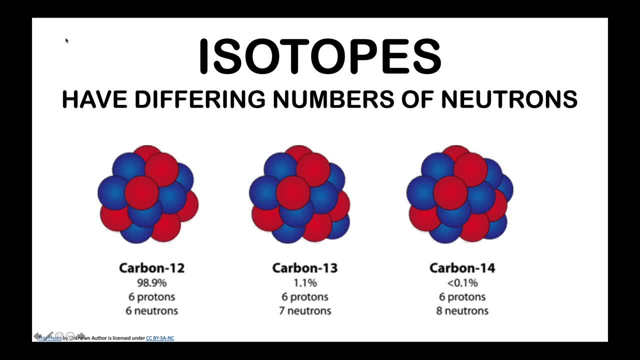 Isotopes are forms of the nuclei of atoms of a particular element that have differing number of neutrons. For example, carbon atoms always have six protons- That's what makes them carbon, And usually carbon atoms have six neutrons too. This isotope is called carbon 12 because 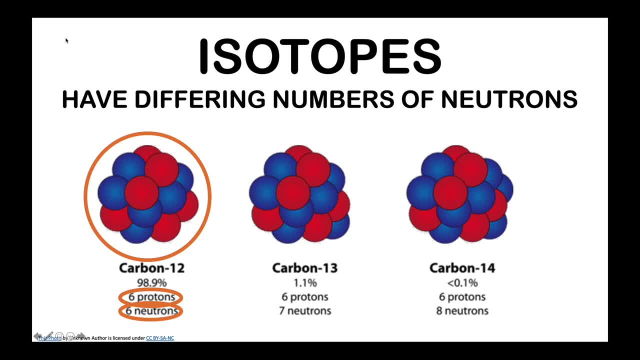 six protons plus six neutrons equals 12 as the total number of particles in the atom In the nucleus. But carbon can also come in other varieties. Carbon 13 is an isotope that contains six protons and seven neutrons, And carbon 14,. 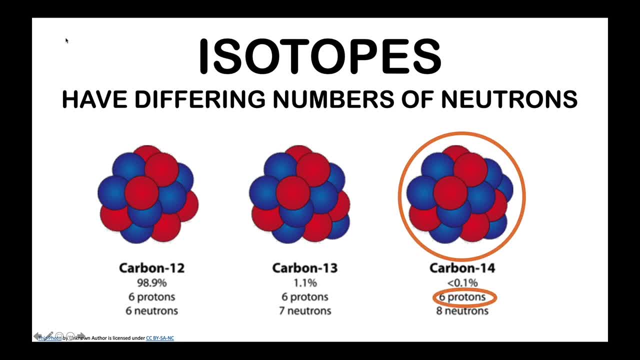 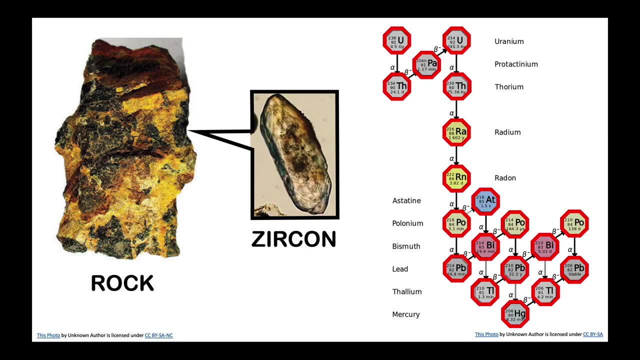 which you might have heard of, has six protons and eight neutrons. These are the three stable isotopes of carbon. You can use isotopes to find out the age of rock And the most well-known type of isotope is radiometric dating. Radiometric dating is uranium to lead dating. This is how it. 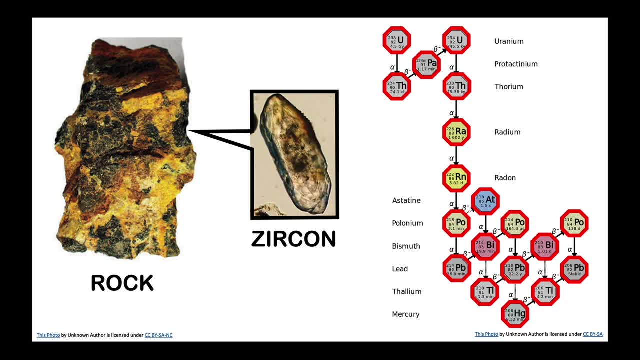 works. You take a rock that you know probably has some uranium in it, usually in a small crystal called a zircon crystal, And, as you can see from the screen, the process is really complicated. Basically, you start with uranium-238. That means there's 238 particles, protons and neutrons in the 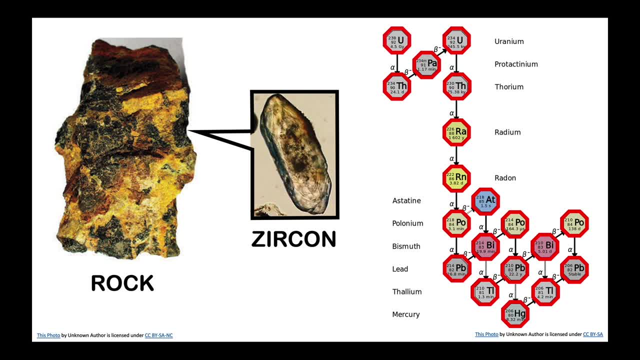 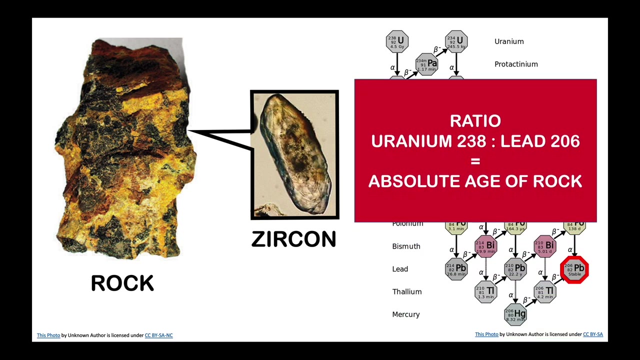 nucleus of this atom. this atom loses both protons and neutrons and slowly turns into something completely different. So it goes through many steps And eventually it ends up being a stable atom, that is lead 206.. Now, if you calculate the ratio of uranium-238, 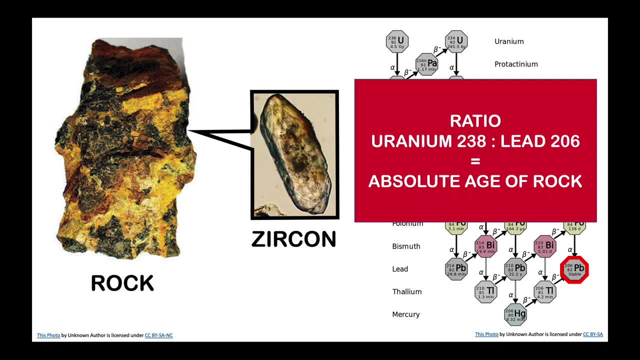 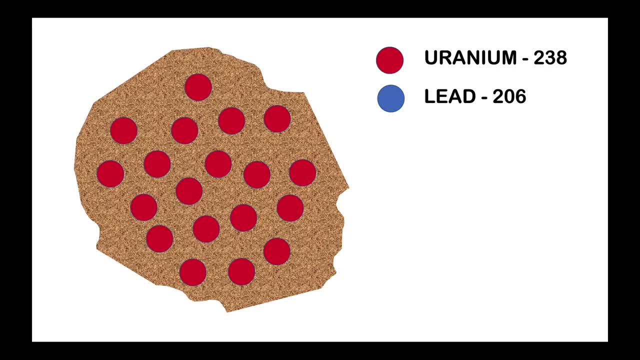 to lead 206 in the rock, you can figure out how long the uranium has been decaying And that gives you the absolute age of the rock. Here's a simpler way of showing it. So the red dots are uranium-238 atoms isotopes. 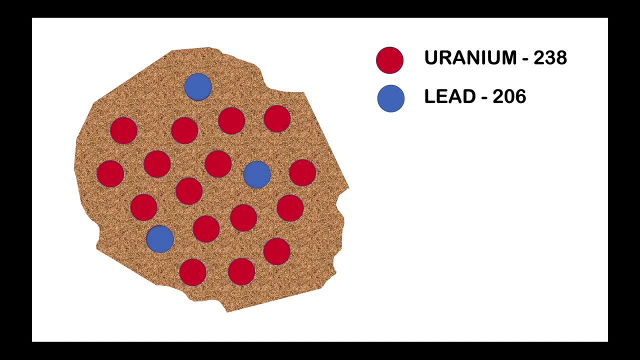 And over time some of them go through that very complicated process and turn into these blue dots which represent lead 206.. You've probably heard the term half-life. The half-life of uranium-238 is 4.5 billion years. This just basically tells you. it takes a really long time. 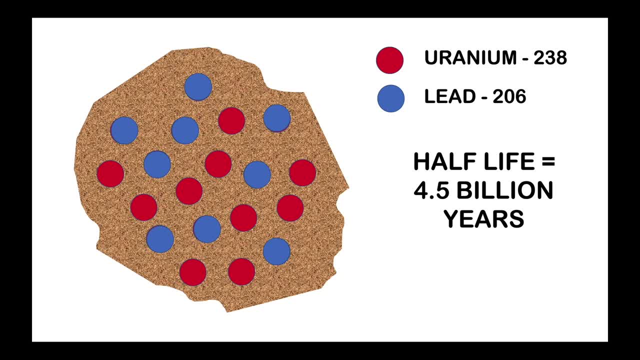 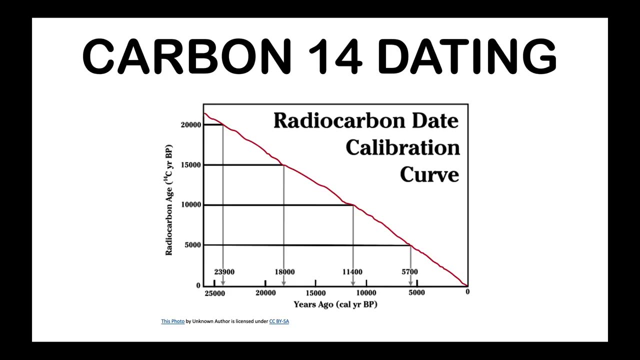 for half of those uranium-238 isotopes to turn into lead 206.. But by knowing how much there is of uranium and lead and comparing those amounts you can calculate the age that the rock has been around. Another type of radiometric dating that you might have heard of: